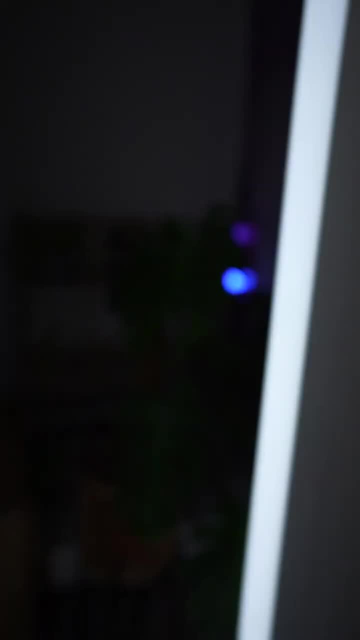 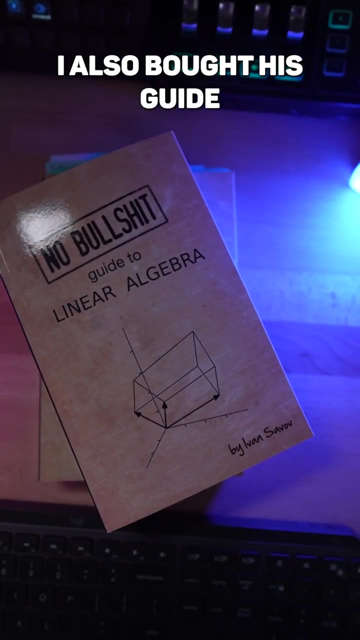 Machine learning books that I've been devouring over the last couple of months. Ivan Savov's Noble Guide to Math and Physics. I found this to be a great refresher to Math Fundamentals. I also bought his Guide to Linear Algebra. Data Science from Scratch by Joel Gruss- First Principles with Python. This is a brilliant. 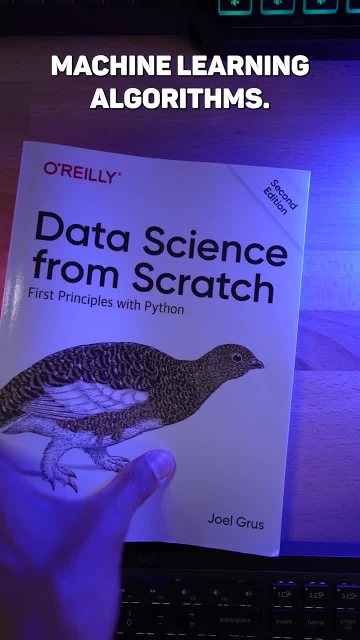 book to understand the nuts and bolts behind some of the most popular machine learning algorithms And, last but not least, DatQuest's Illustrated Guide to Machine Learning. A triple bam These. 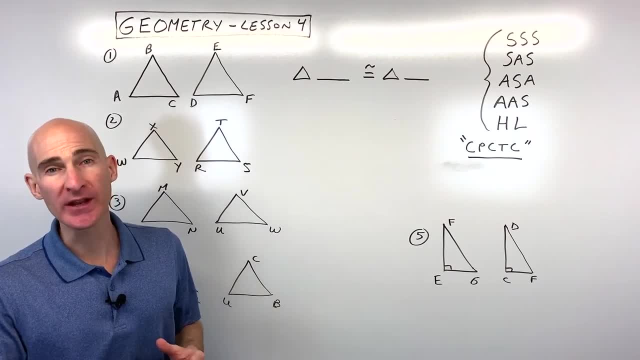 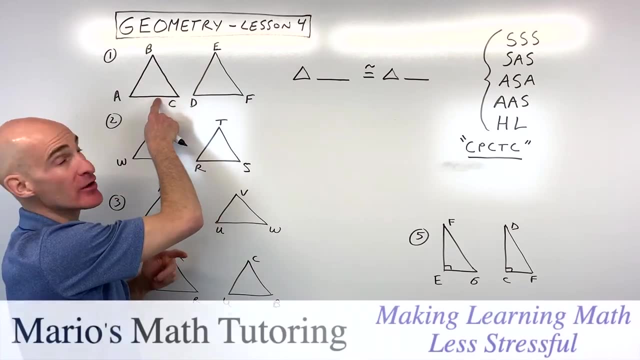 In this lesson, you're going to learn how to prove triangles congruent. Now, when we talk about triangle congruence, what we're referring to is if I were to take some scissors and cut out this triangle here, place it on top of this triangle here, if everything matches up, meaning the 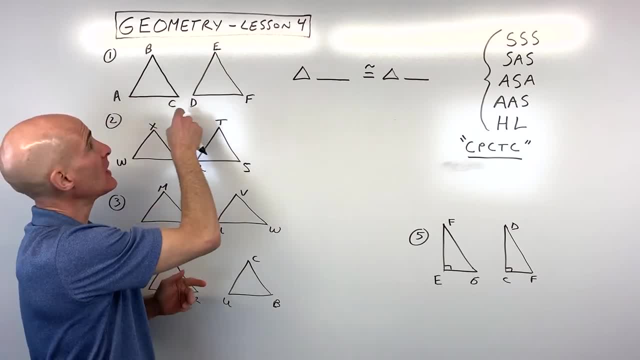 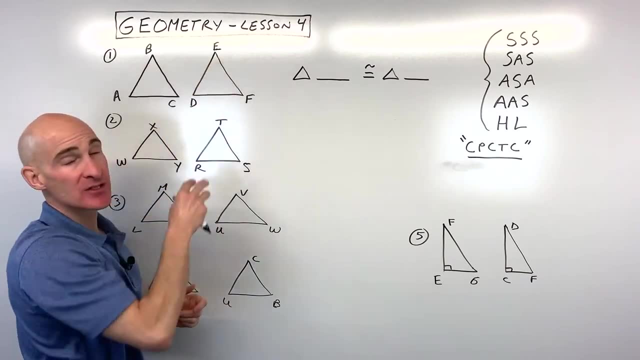 corresponding sides or the sides that match up are all congruent, and the corresponding angles: okay, those all match up and those are all congruent. then we say that this triangle is congruent to this triangle and we can write what's called a triangle congruence statement. 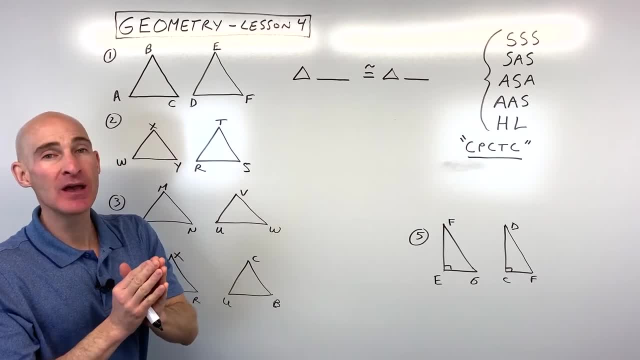 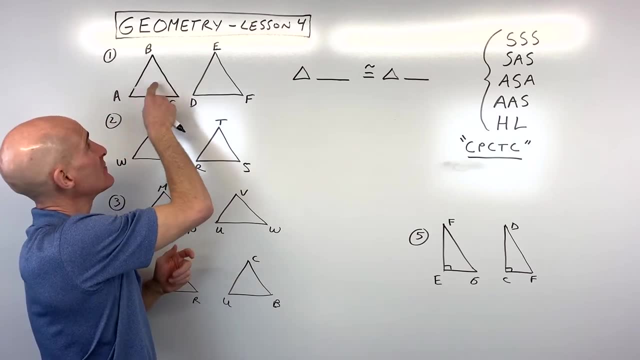 So congruence just means that you know they're exactly equal, they exactly match up. Now the thing is, a triangle actually consists of six pieces. right, It consists of three sides, it consists of three angles, so a total of six components. But what we're going to be talking? 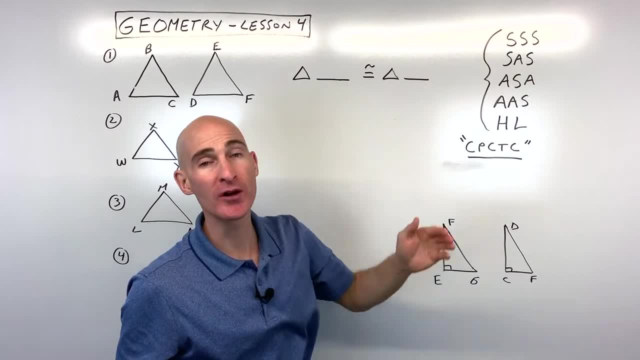 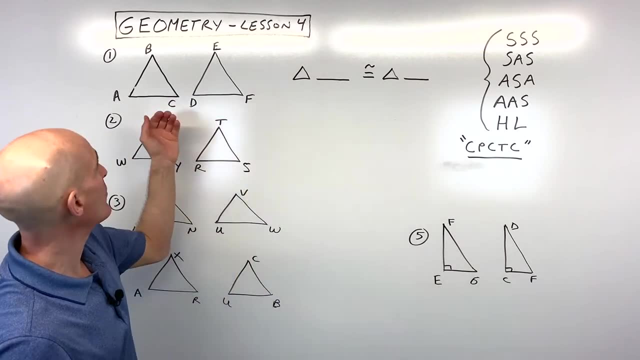 about in this video is that you can actually prove triangles congruent by showing specifically three components are congruent, and that's what we're going to talk about now. So the first thing we want to look at is how to prove triangles congruent using the side-side-side.